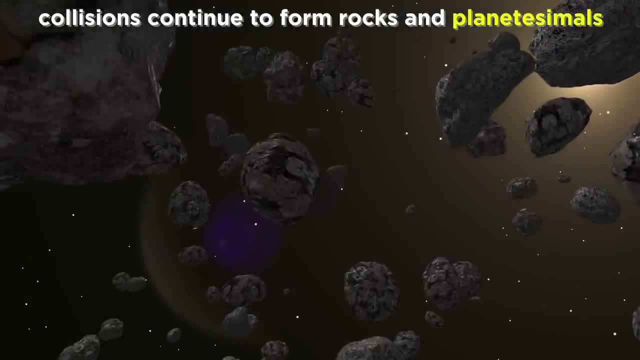 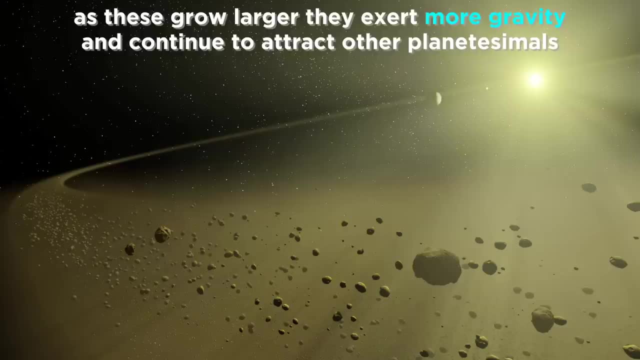 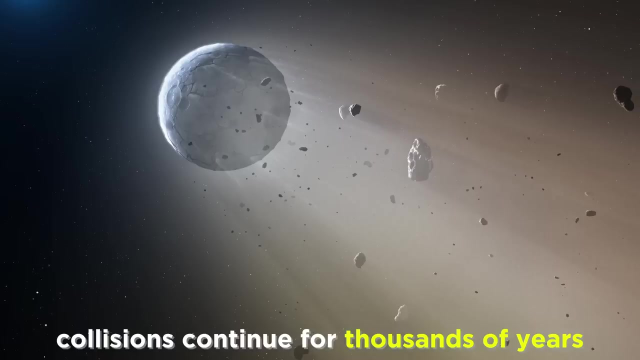 These larger pieces continued to collide with others to form rocks And then larger objects called planetesimals, increasing their gravitational influence as they grew, eventually attracting other planetesimals. Over hundreds of thousands of years, all of these clumps of rock and ice continued to 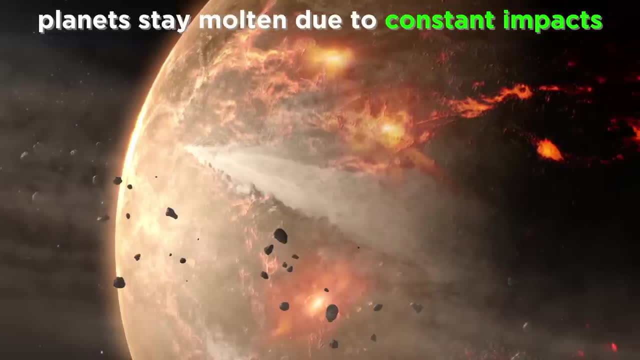 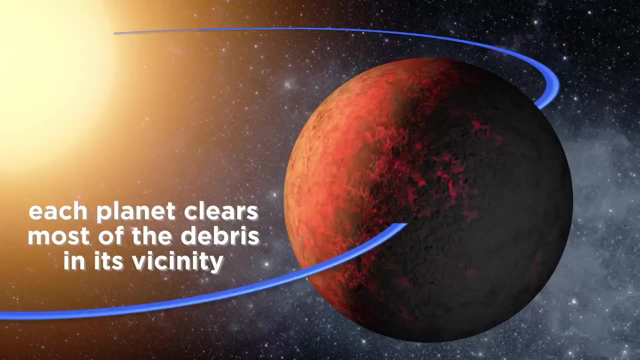 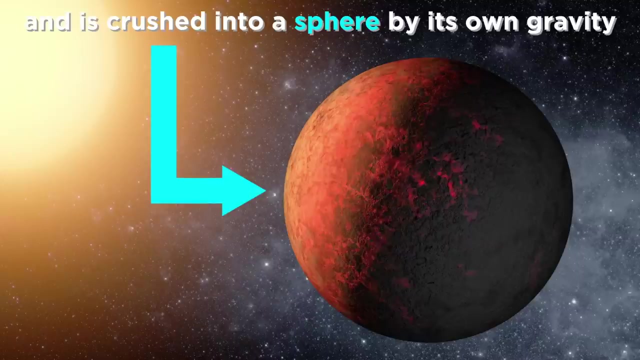 collide and accumulate with every impact, generating lots of heat, keeping things relatively molten. As most of the surrounding debris at each particular orbital distance was cleared, the objects became massive enough to take on a spherical shape under the influence of their own gravity. 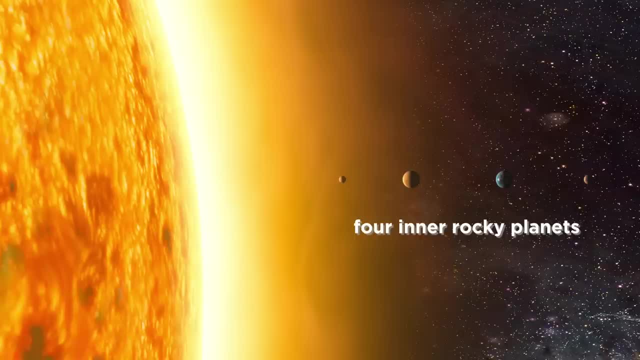 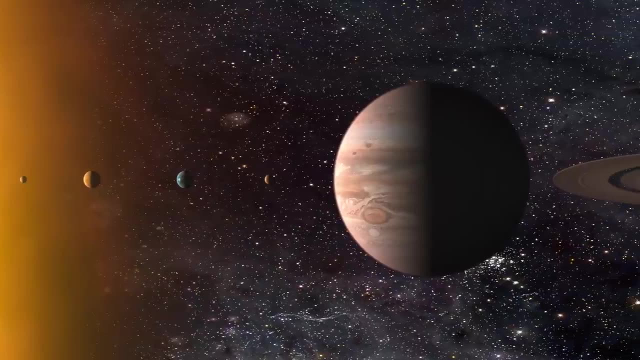 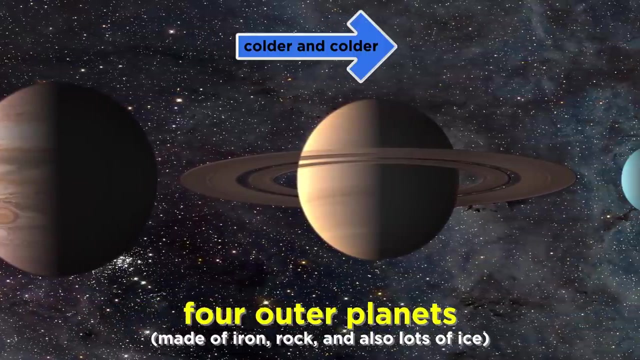 These are the inner rocky planets we know today For the gas and dust that made up the outer regions. this also collected into spheres due to gravity, though, beyond just iron and rock, these also contained lots of ice, given the colder temperatures present at this greater distance from the sun. 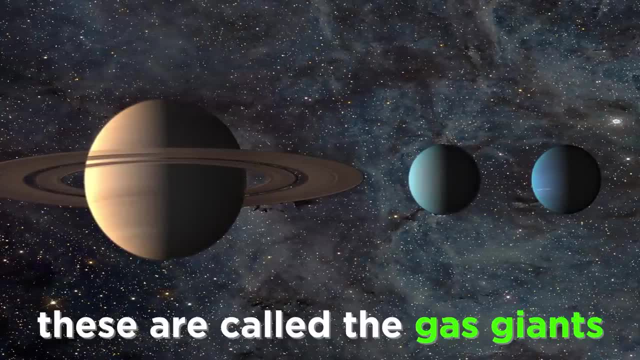 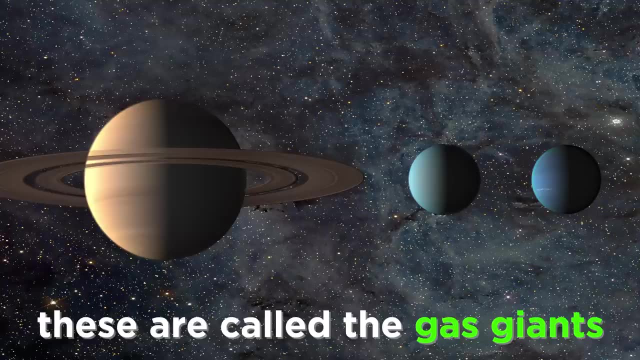 So these objects became massive enough to take on a spherical shape under the influence of their own gravity. Once large enough, they could also attract much of the gas in their vicinity. so these became the gaseous planets we call the gas giants. 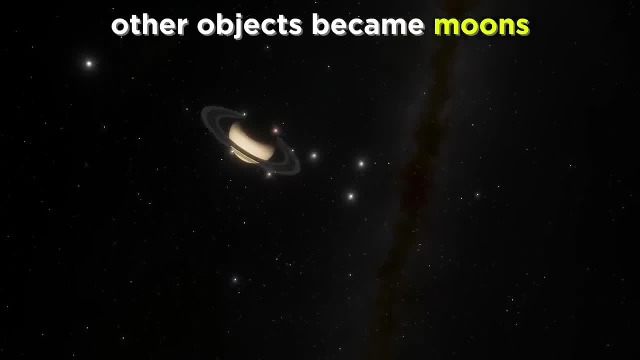 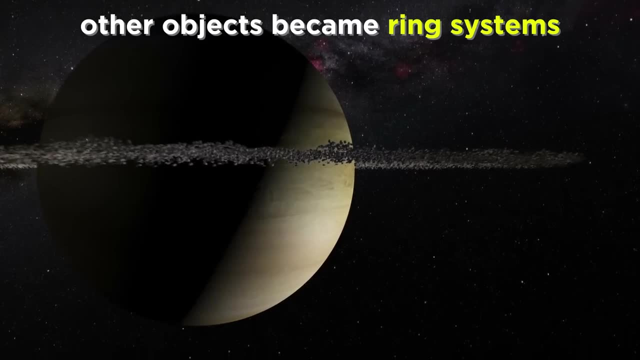 Planetesimals that didn't make it into a planet accumulated into moons or remained in the form of smaller objects like asteroids and comets and other loose matter collected into rings around the larger planets, And thus the solar system was born. And thus the solar system was born. 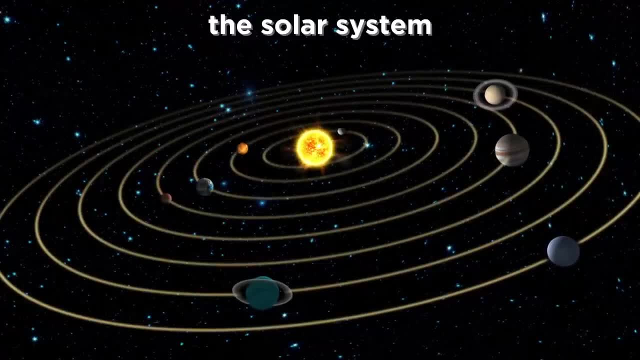 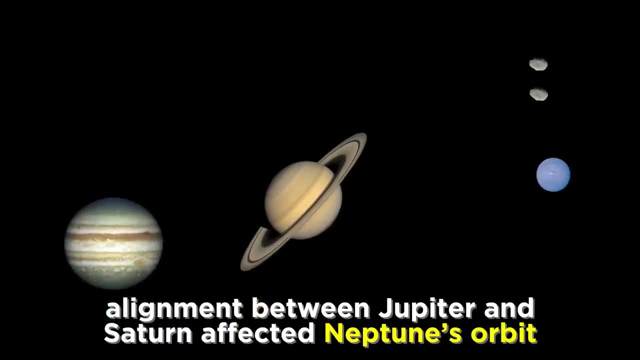 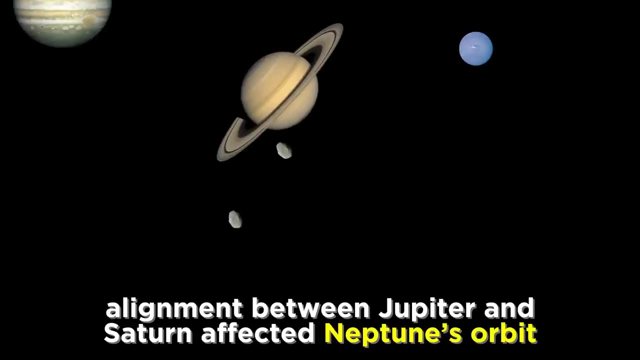 Things have not been completely static since this formation. Objects are jostled around all the time, like a few billion years ago, when Jupiter and Saturn lined up in such a fashion that Neptune's orbit altered in turn, sending small objects in the outer solar system towards the inner planets, raining down on them in an event. 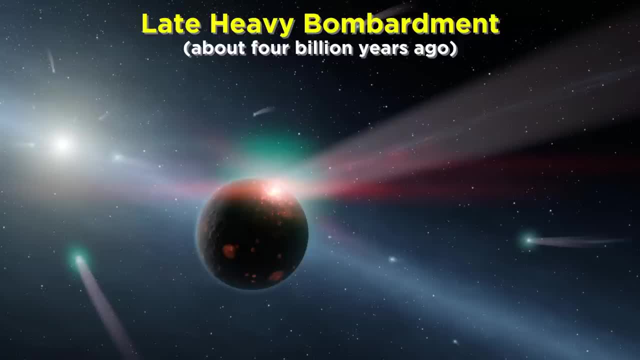 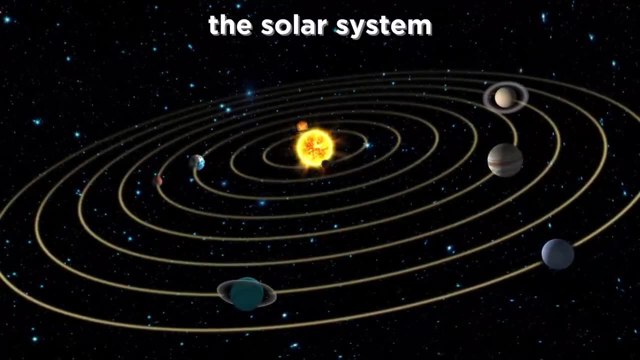 called the Late Heavy Bombardment. But for now, let's focus on the solar system as we see it today. But for now let's focus on the solar system as we see it today. Later in the series, we will devote an entire chapter to each major body in the solar system. 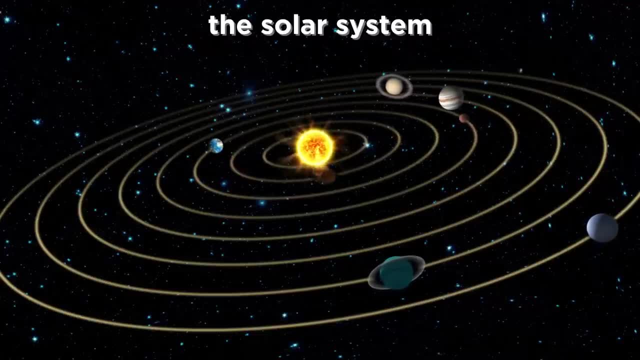 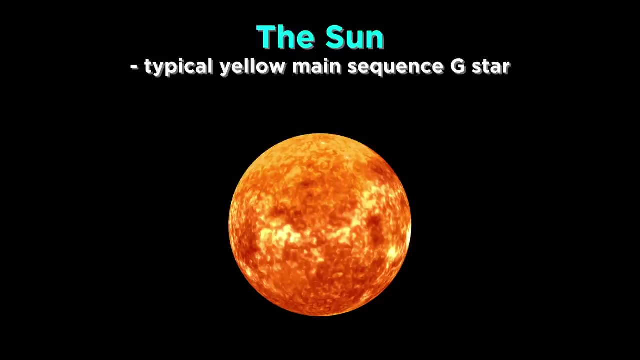 but let's just briefly describe some of these objects right now. First, there is the sun. This is a typical G star, a yellow main sequence star. as we mentioned, It is a population one star, as it is relatively new, having formed from a cloud of gas and 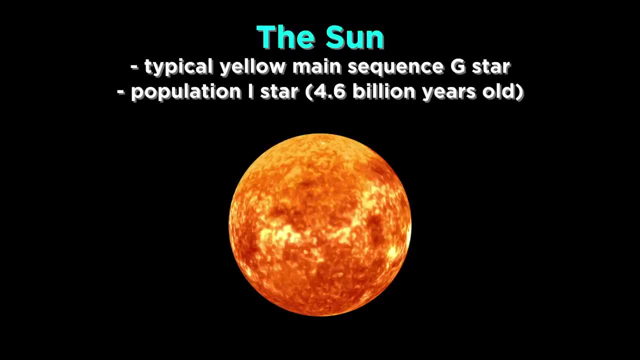 dust, which contained significant amounts of material that had been ejected from the sun. It is a population, one star, as it is relatively new, having formed from a cloud of gas and dust, which contained significant amounts of material that had been ejected from the death of other older stars. 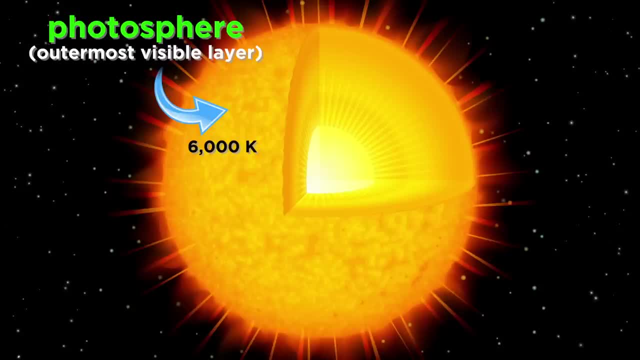 Its photosphere, or outermost visible layer, burns at around 6000 kelvin, while the hot inner core burns at around 15 million kelvin, unfathomably dense because of the crushing gravity, but still remaining a plasma due to the heat. 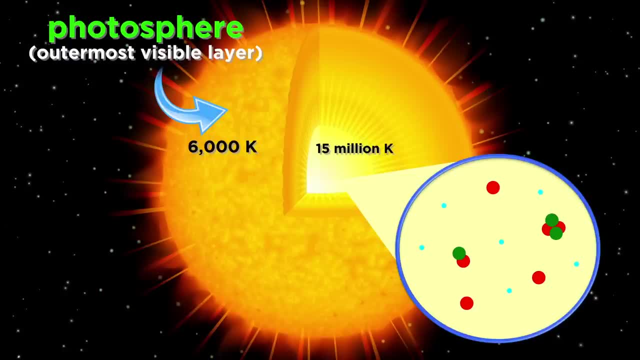 This is a state of matter beyond the gaseous state, where it is too hot for electrons to be coordinated to atoms. So it's just a supermassive state of matter. So it's just a supermassive state of matter. So it's just a supermassive state of matter. 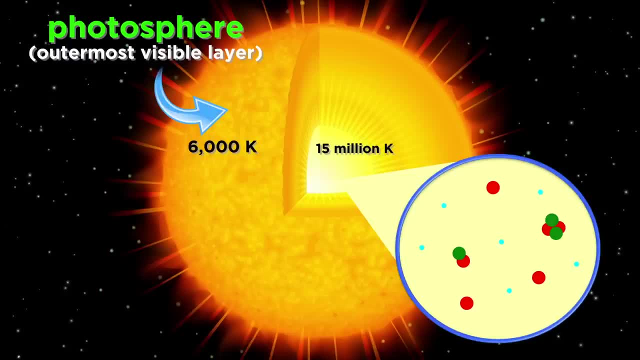 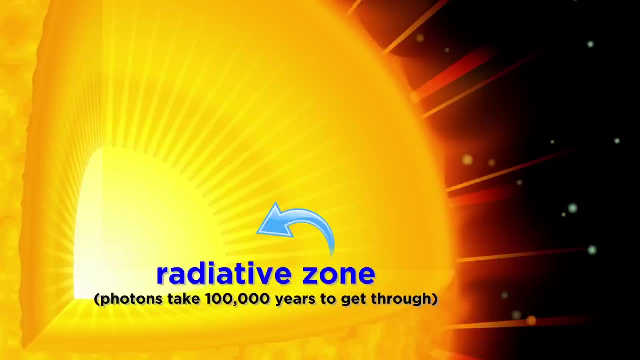 It's a type of nuclei and free electrons whizzing about In between the core and the photosphere is a radiative zone where photons radiate outwards, absorbed and emitted in random directions for a hundred thousand years before they eventually find the surface and can move through space. 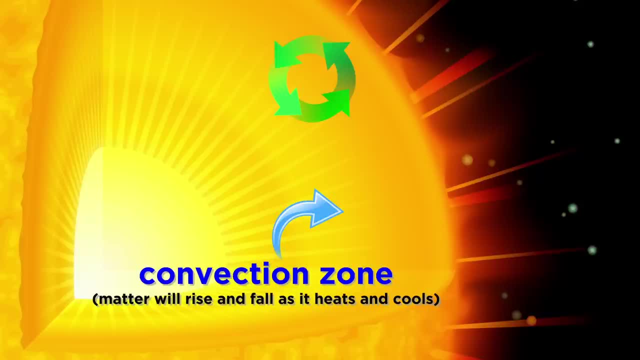 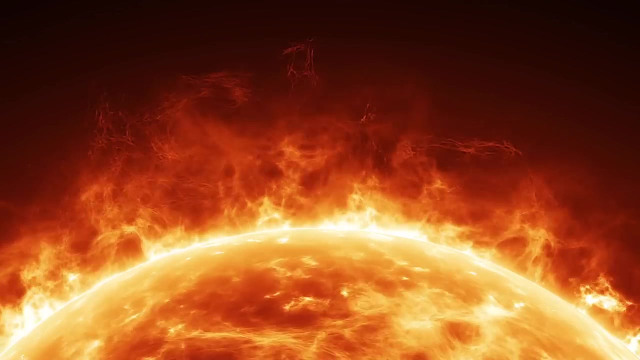 There is also the convection zone, where material is far enough from the core that it has an opportunity to cool as it rises, which allows it to sink back down, where it then heats back up, continuing in a cyclical manner. It may come as a surprise that the sun also has an atmosphere. 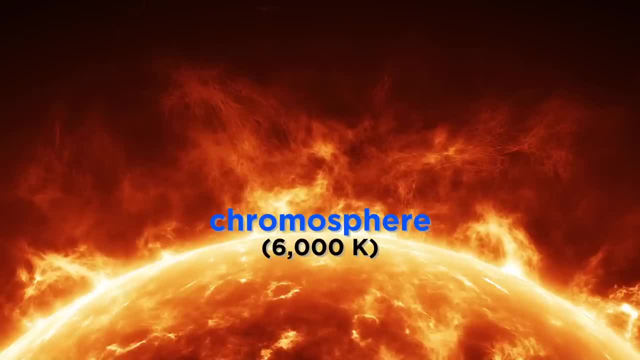 The lower atmosphere is called the chromosphere, which is relatively cool, and the outer atmosphere is called the corona, which strangely jumps back up to a million kelvin. We still don't fully understand how this material can be so hot, though it is widely. 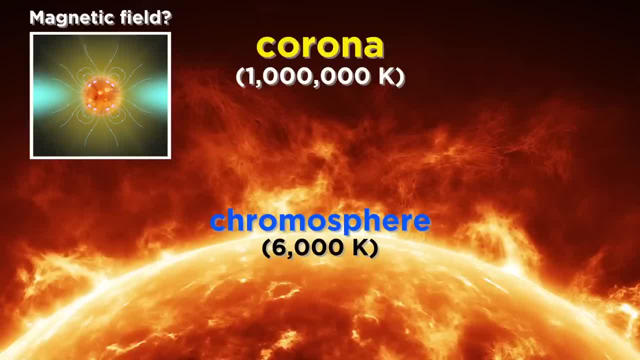 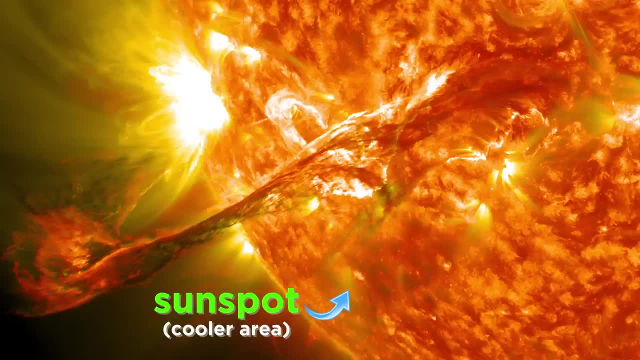 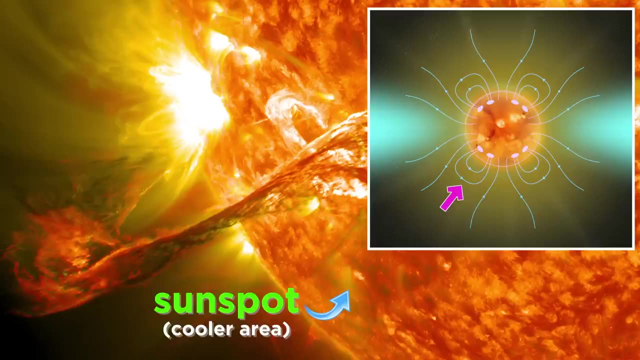 agreed that the sun's magnetic field is hot. It is somehow involved, while some propose that it is acoustic energy that is responsible. Along the surface of the sun, we can find dark patches called sunspots, which is where the magnetic field lines loop out of the sun, preventing the rise of gas in particular locations. 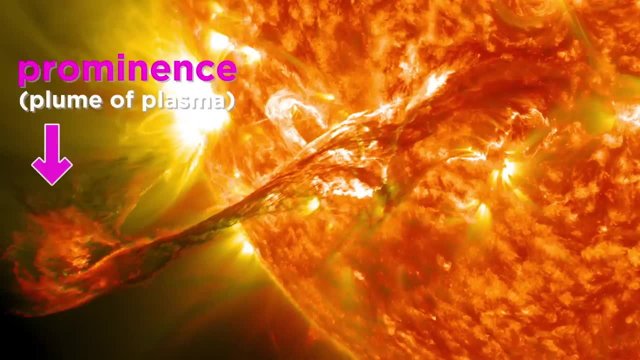 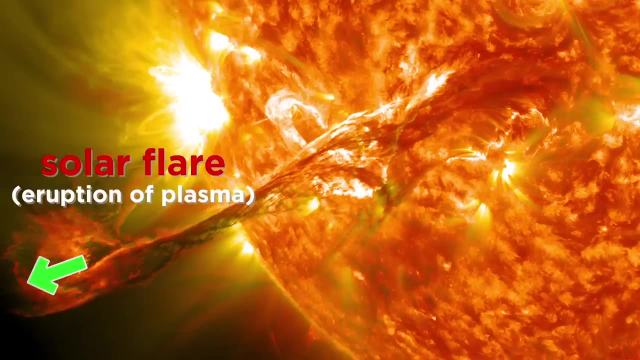 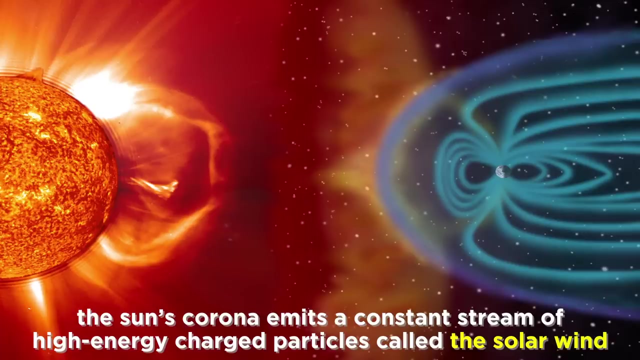 and thus generating cooler, darker areas. In addition, there are plumes of plasma called prominences, which are also generated by the magnetic field. The field can also produce sunspots. In addition, there are solar flares, which are eruptions of hot plasma in the chromosphere. 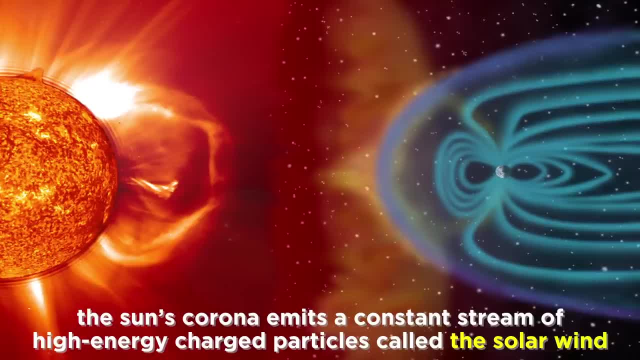 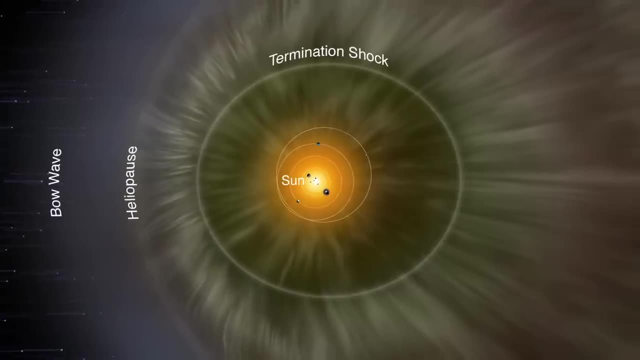 Beyond flares, activity in the corona results in the solar wind, a constant stream of plasma or high-energy charged particles flying through space in all directions. This solar wind travels for incredible distances, the limit of which marks the end of the heliosphere. 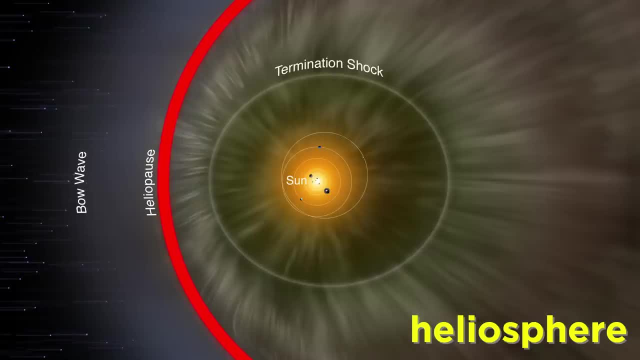 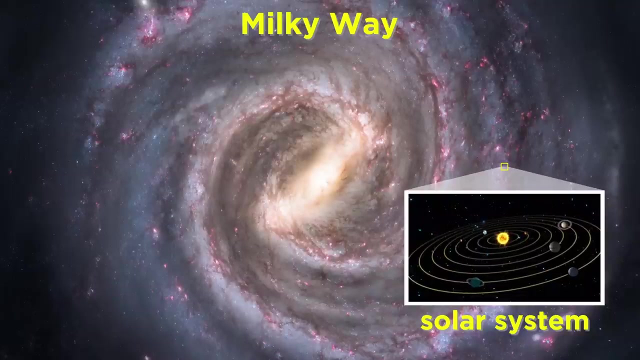 This boundary for the solar wind is the limit of the sun's influence on its surroundings, which means it qualifies as the boundary of the solar system itself, lying extremely far beyond the outermost planet Relative to the Milky Way, the solar system is miniscule. 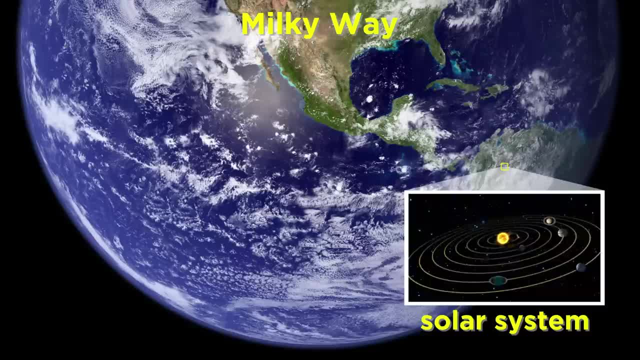 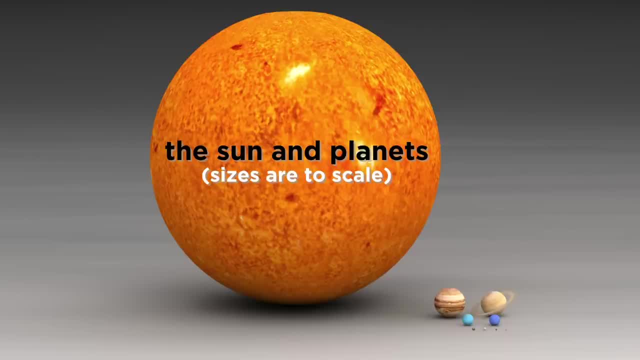 If the galaxy were shrunk down to the size of the Earth, the solar system would be the size of a pancake. But to now look at the solar system as a whole and all the objects in it, we see that, relative to the planets, the sun is absolutely immense. 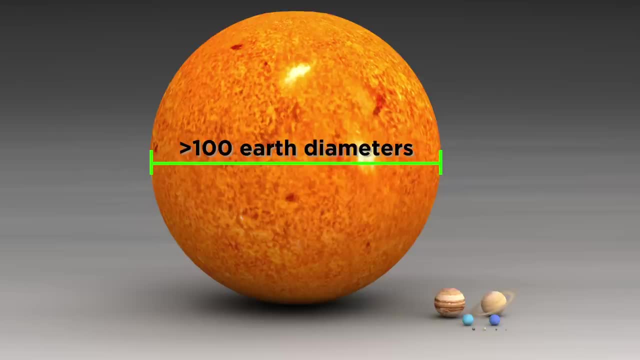 Its diameter is more than a hundred times greater than that of the Earth, which means it would take over a million Earths to fill up the sun. The sun makes up about 99.86% of the mass of the solar system, so it really calls the. 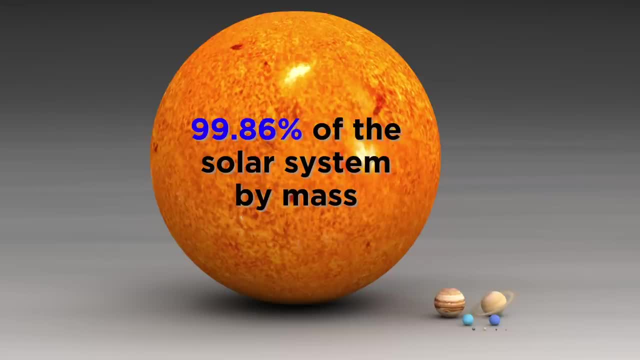 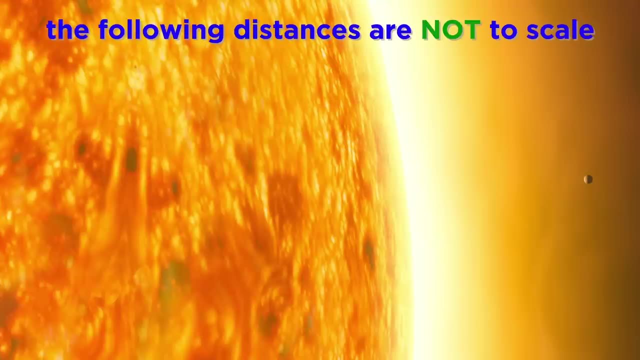 shots, and most of the planets maintain near-circular orbits around it. Let's quickly mention these planets in their order from the sun. Bear in mind that any illustration of the solar system is nowhere near to scale, as the planets are incredibly far apart, but we can use this to simply familiarize ourselves. 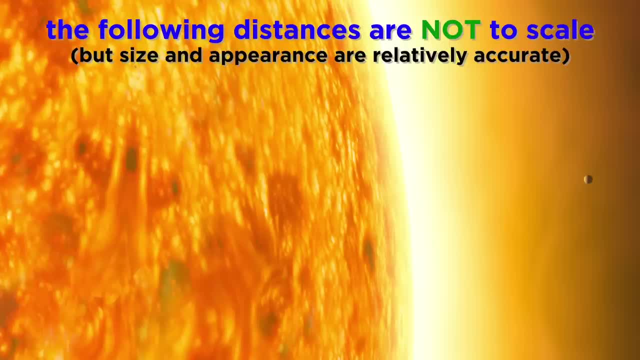 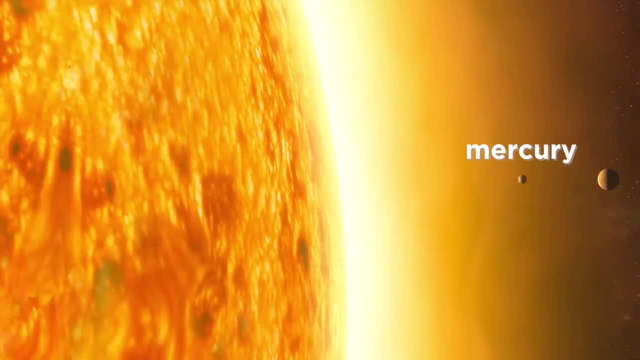 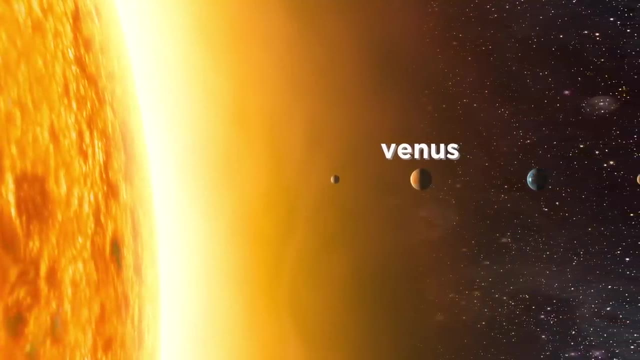 with their names and approximate relative sizes, as well as their appearances and general features. First is Mercury, the barren planet closest to the sun. Venus is next Hot, Heavily volcanic, A hellish world. Then the third rock from the sun, our little Earth, home to everyone you've ever met. 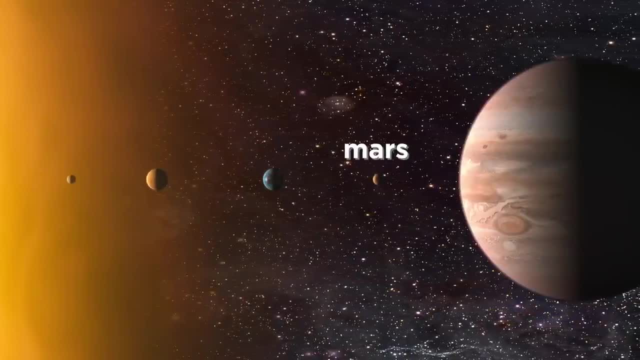 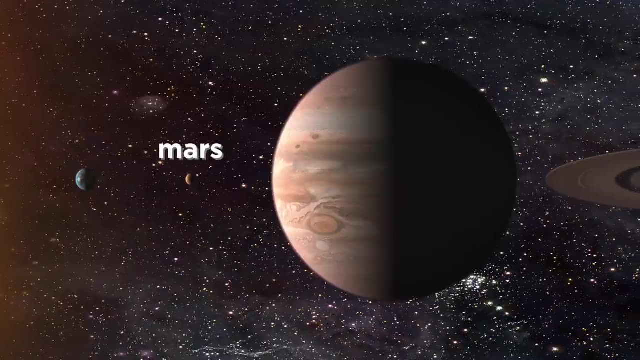 and every place you've ever gone Just a bit further is Mars, the red planet where humans will likely set foot very soon, making history in the process. Next is the asteroid belt, which is not shown but will be discussed later. 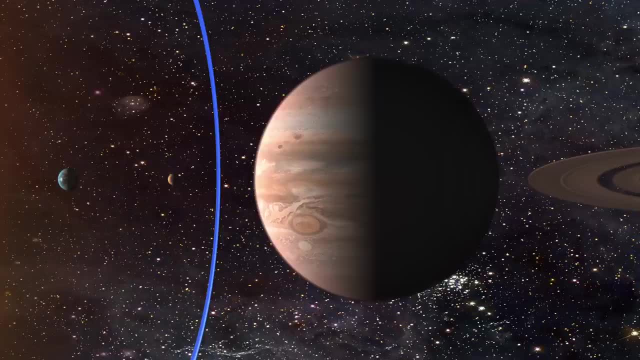 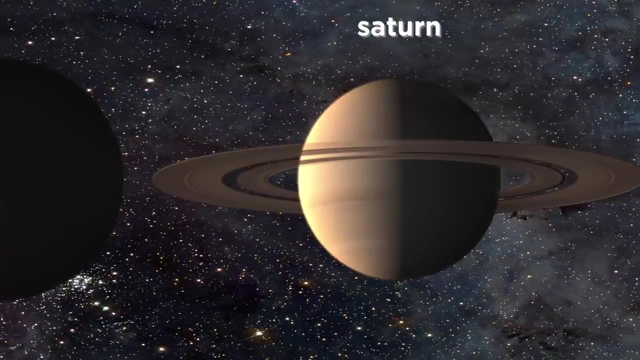 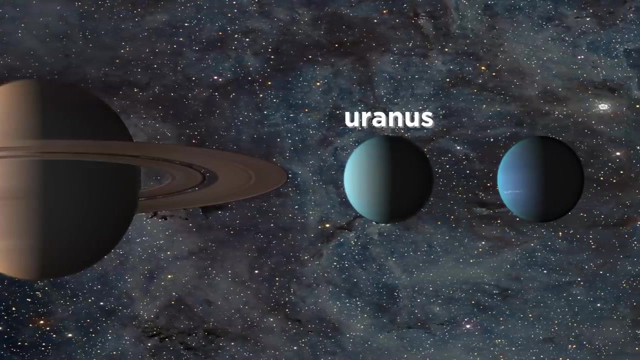 And that marks the end of the inner rocky planets. The first of the gas giants is Mars. The second of the gas giants is Jupiter, the largest of the planets. After that comes Saturn with its breathtaking system of rings. Then comes the icy planet, Uranus. 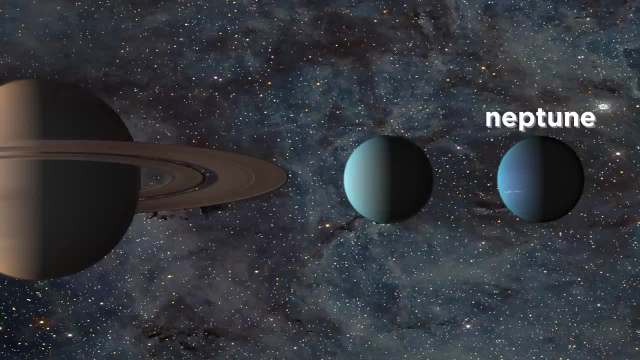 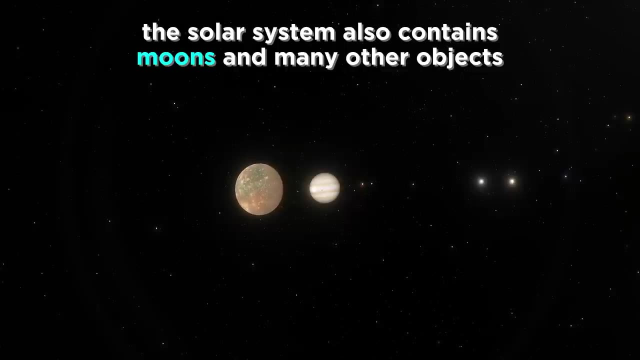 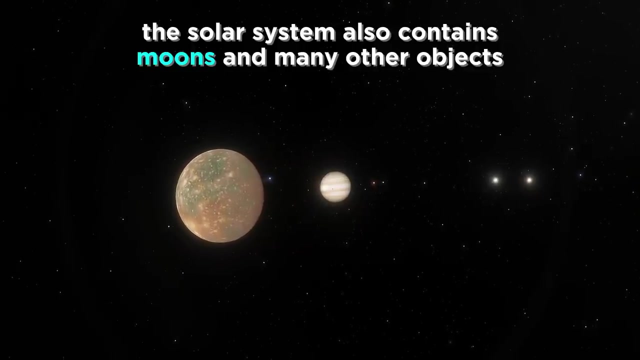 And lastly, the outermost planet, Neptune, Four small balls of rock and four big balls of gas. Most of these planets have moons, and there are lots of other objects in the solar system that are worth discussing, But we will get to all of them a little later in the series. 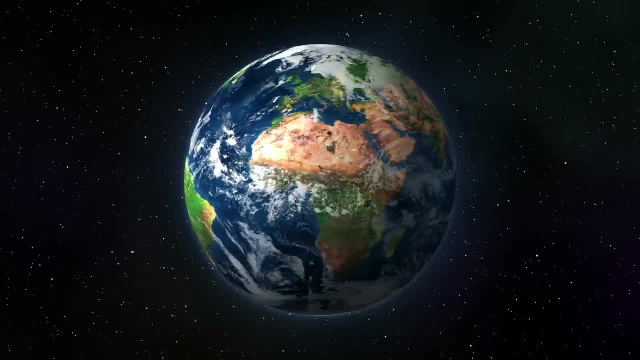 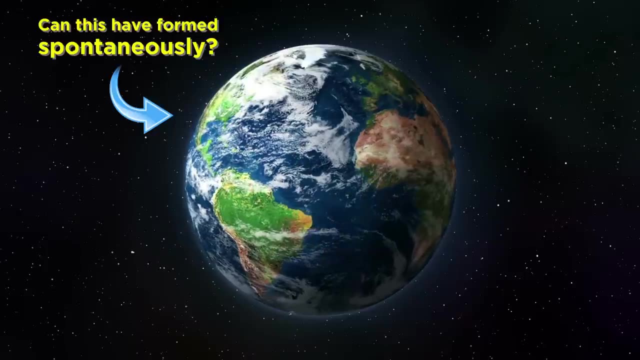 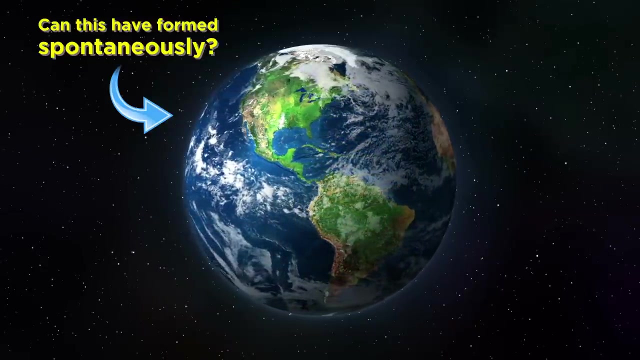 So we can see how at first glance it may seem impossible for objects as complex as Earth and the other planets to form spontaneously. but even with just a rudimentary understanding of only two astronomical processes, solar system formation becomes quite intuitive or even obvious. 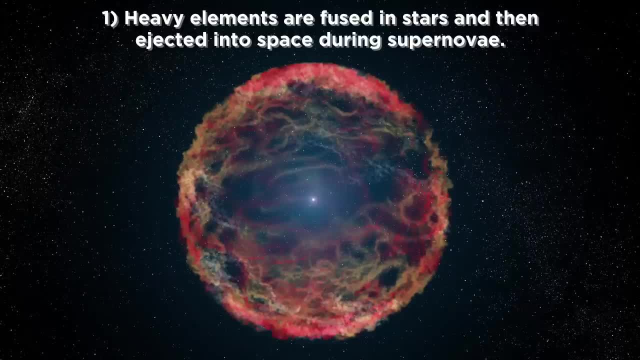 The first of these processes is the fusion of heavy elements inside the atmosphere. This is where we find the most interesting part of the solar system. The most interesting part of the solar system is the fusion of heavy elements inside a huge, high-mass stars, which are then ejected into the interstellar medium during a 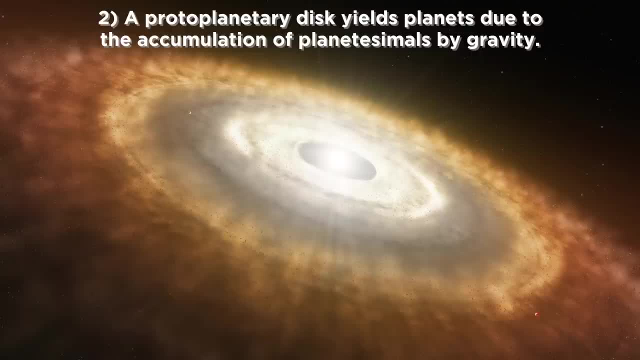 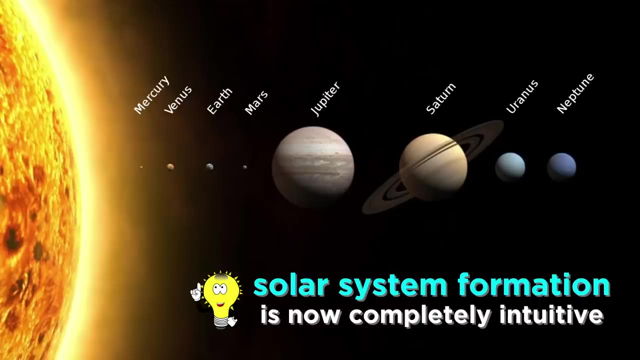 supernova. The second is the accretion of interstellar gas and dust to form a protoplanetary disk, which then slowly accumulates into large spherical objects at varying orbital radii, purely by gravity. Now the spontaneous formation of the solar system makes just as much sense as any other knowledge we can. 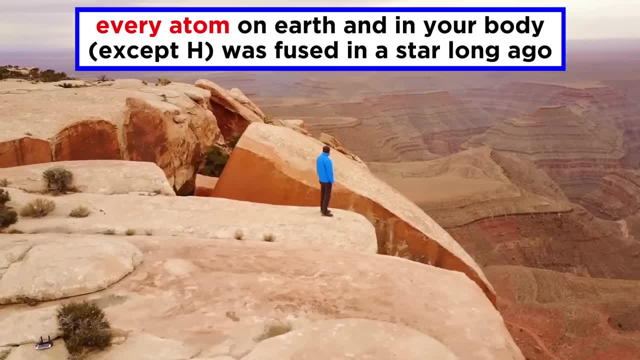 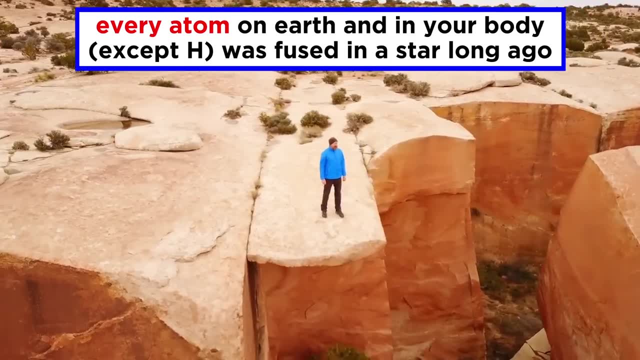 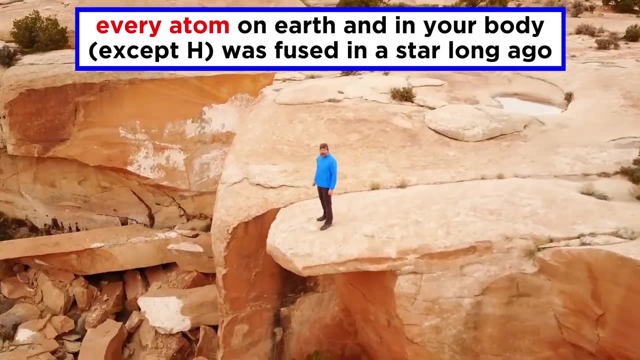 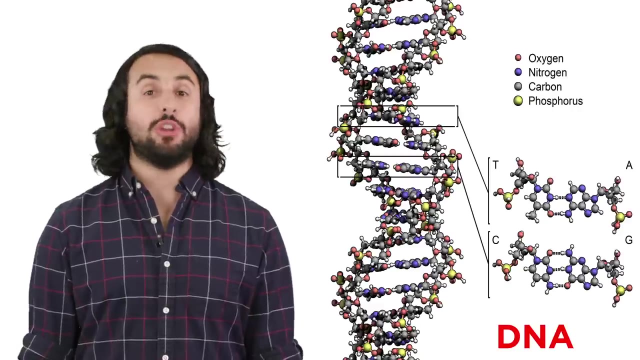 infer from our immediate surroundings. We also come to the incredible realization that every single atom on Earth, and therefore every single atom in your body other than hydrogen, was fused inside a long dead star: All of your carbon, oxygen, nitrogen, phosphorus and all the trace metals that make you what